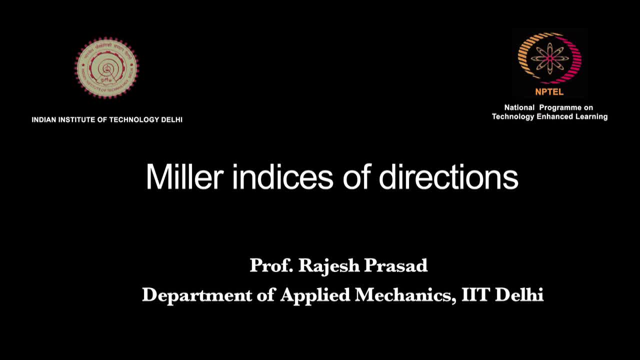 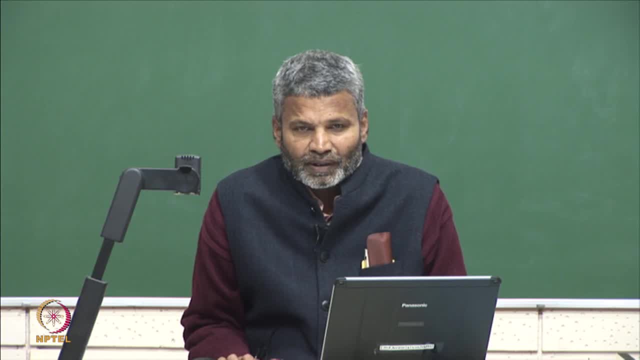 Hello, today we will start a new topic. Till now we have been discussing Bravais lattices, 14 Bravais lattices and 7 crystal systems. We looked how symmetry helps in classification of crystals into these schemes. We will now start a new topic: the Miller indices of directions. 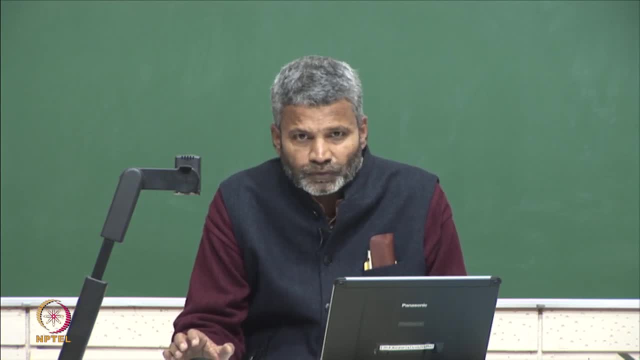 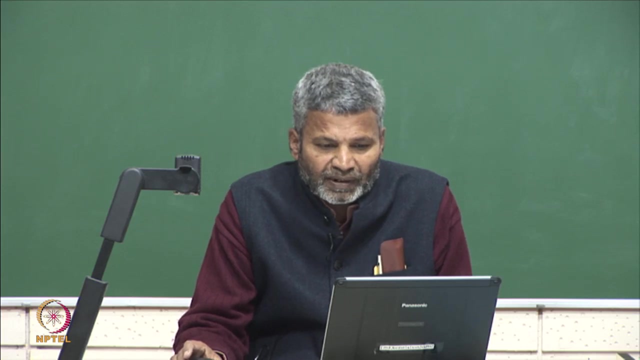 and planes. These are techniques or tools to specify various directions as a when we work with crystals, we need to specify or name different directions and planes in a crystal. So Miller indexing is an standard method which has been, which is being used for this purpose. So let us we will first, in this video, we 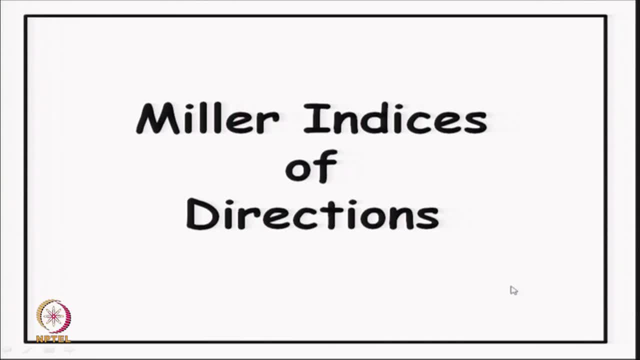 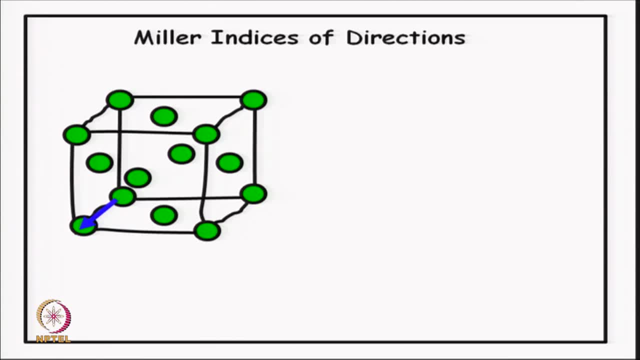 will look at Miller indices of directions and in the next one we will take Miller indices of planes. So let us look at Miller indices of direction. Suppose we have this crystal, a unit cell is shown a face centered cubic lattice. So all these large circle are the lattice points. 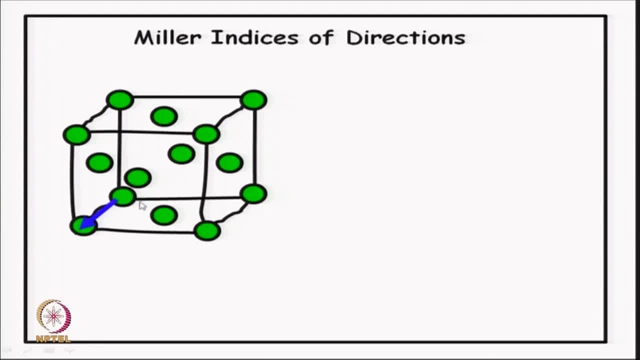 and we want to specify a certain direction. Let us say this blue direction edge of the cube. Of course the cube has this edge. it has this another edge, two horizontal edges and one vertical edge. So I have picked out one of them, this blue one, and I want to give 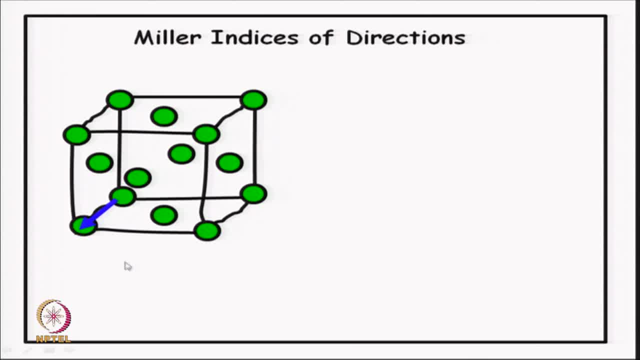 a name to it. Of course, in common is: I can say that it is the edge of the cube on its bottom face coming out of the screen, so to say, And this one is an edge line, So this lying in the screen and this is a vertical edge, and so on. 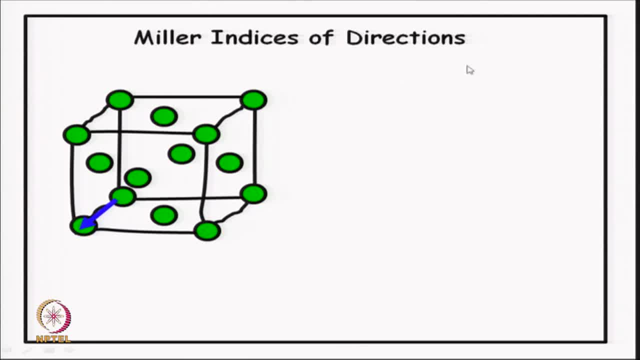 However, Miller indexing will give us a specific notation or a specific system to name this blue line. So let us look at how we do that. we will go step by step. The first step in Miller indexing is to choose an origin. on the direction: 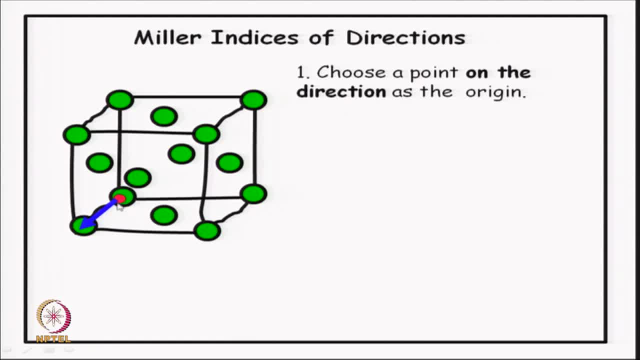 So I have chosen this back corner as my origin pointed out in red. So the first step is always to choose the origin, and I have highlighted here that on the direction. So the origin always has to be on the direction. it should lie on the direction or vice versa. 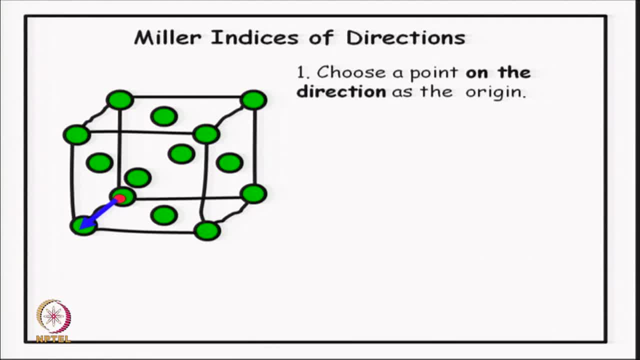 The direction should pass through the origin, or origin should be so chosen that it lies on the direction. This freedom of choice exists in crystallography. In the crystallographic coordinate system. we are free to choose the origin anywhere we wish. So if I want to index this blue direction, I choose the origin on the blue direction. 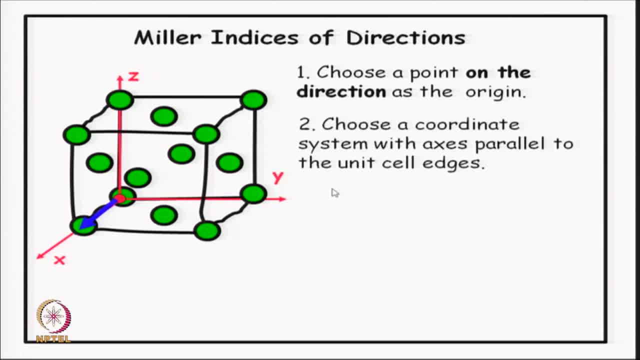 and I took this point as the origin. The next step Is to choose a coordinate system, crystallographic coordinate system with axes parallel to the unit cell edges. So in this case I have chosen x, y and z, with the 3, x, y, z directions parallel to the unit. 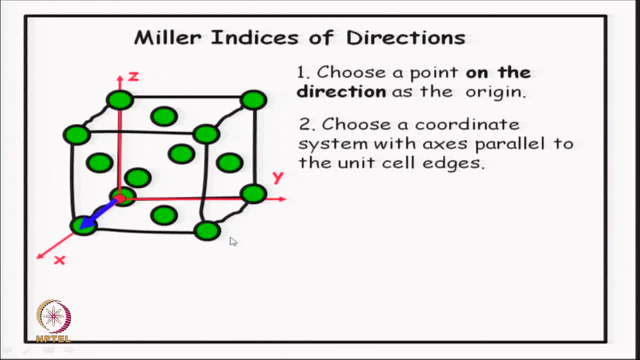 cell edges. Here I have read for illustration purpose: I have taken a cube. even in a non cubic crystal. even if the angle between x and y is not 90 degree And even if z is not perpendicular to x and y, we will always choose our x, y and z parallel. 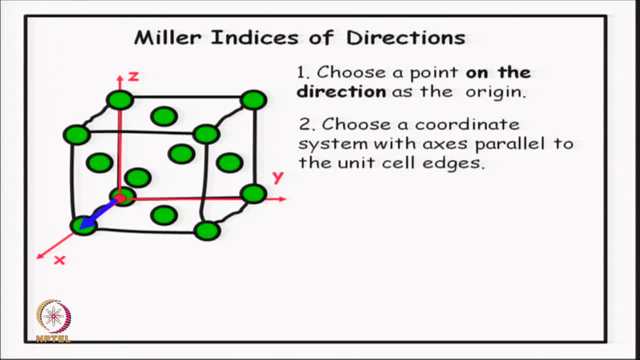 to the unit cell edges. This is what is called the crystallographic coordinate system. So we will be using the crystallographic coordinate system with unit cell edges as our axes. So we have done that for this direction. Now The next step is to find the coordinates of another point on the direction, in terms of 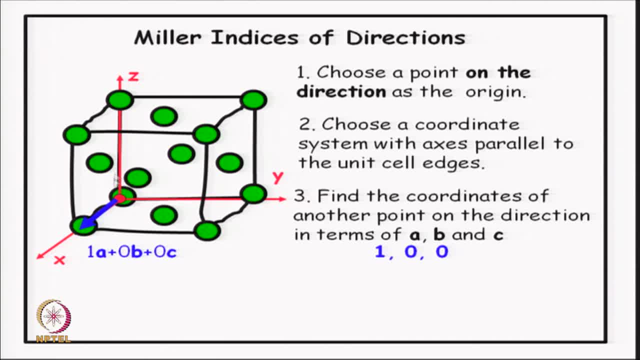 a, b and c. A, b and c are the 3 lattice parameters, So in this case they are the edge lengths. So a is the edge length of the unit cell along the x axis, B is the edge length of the unit cell along y axis and c is the edge length along the 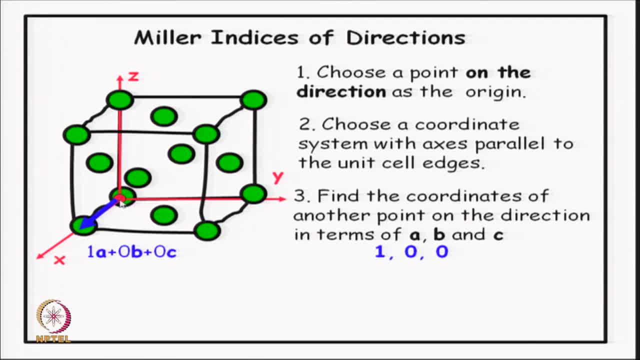 z axis. So in terms of these 3 vectors, the a, b and c vectors, I will now try to express the blue vector, which is the vector of my choice direction of my choice, and in terms of these 3 vectors. So here it is very simple. 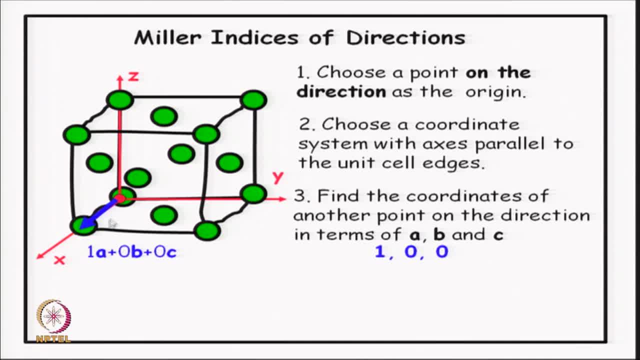 It is 1 times a because the direction is along the x axis and it is of the length equal to a. So it is one times a, 0 times b and 0 times z. Now let us see. Is there any problem? Yes, 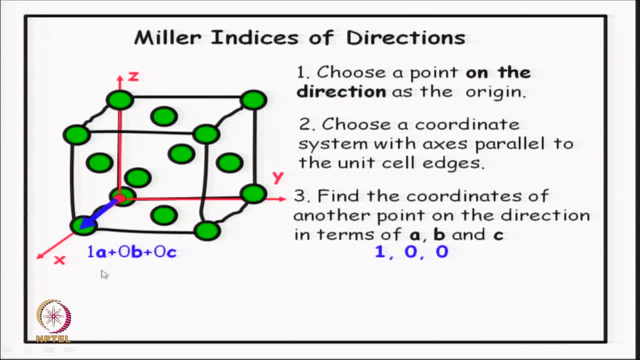 c. So I just take these coefficients 1, o, o to represent this direction. So I find the coordinates of another vector in terms of a, b and c. So the first one means 1 times a, the second, 0, means 0 times b and then 0 times c. 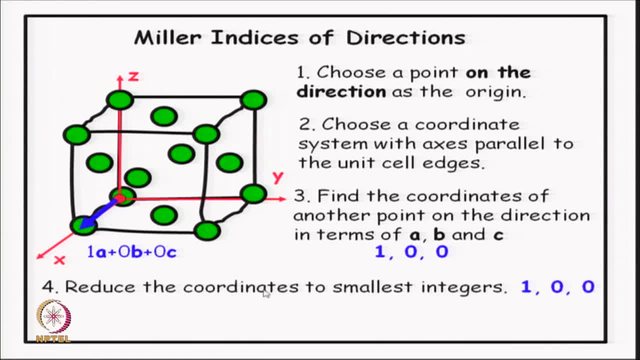 The next step- which in this case is redundant, but we will write it out because we will use it in the next example- is to reduce the coordinates to smallest integers, and this can be done either by dividing by a common factor or multiplying by a common factor. So suppose we had fractions. 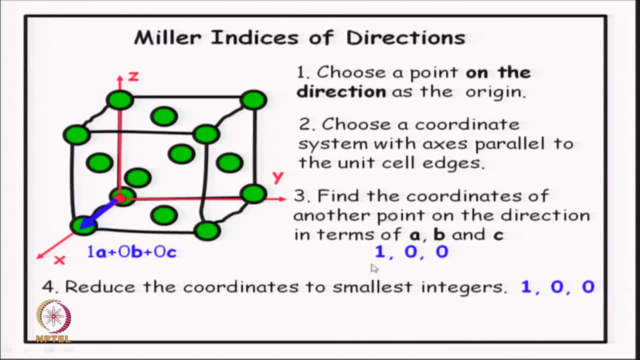 then we will multiply by some common factor such that the fractions get cancelled. or suppose if we had a common factor In all these three, then we will divide by that common factor to cancel out the common factor. So this is a step of reducing the coordinates to a smallest integers In this. 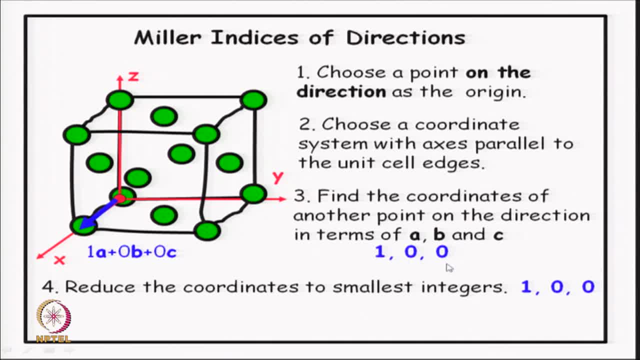 case, nothing is required. 1, 0, 0 is already a smallest integer, so we carry on with that. And then the final step is to just put these three numbers in a square bracket. This is an important step. A square bracket is not my choice. 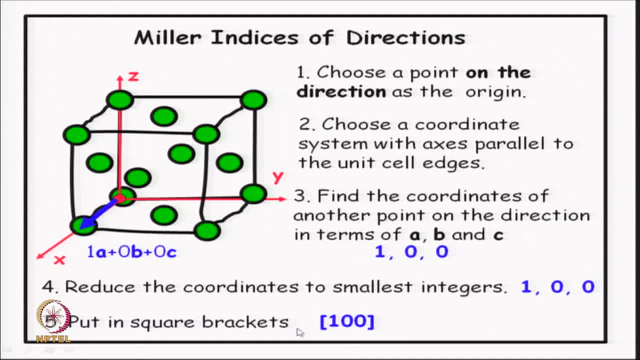 In this presentation or this slide. it is an internationally agreed upon convention that directions will always be represented by numbers inside a square bracket, So we will follow this convention. So 1, 0, 0 is the direction which is represented by this blue line. 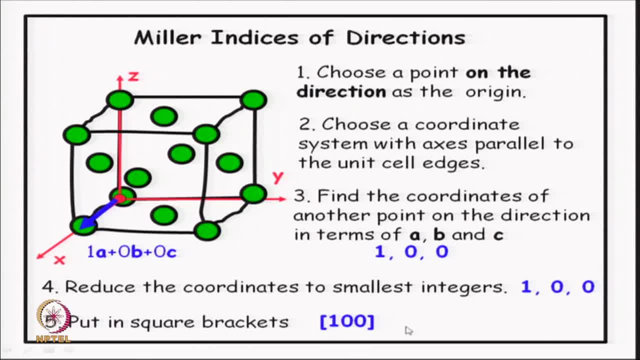 So 1, 0, 0. there is a slight difference between vector terminology and the Miller index of a direction, Although I picked up one vector, this blue vector, to along this line and used that to calculate my Miller indices. Once I have find the Miller indices- 1, 0, 0, it is 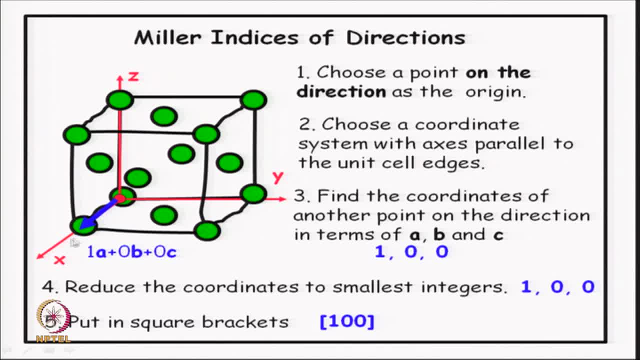 not representing just this blue vector but this entire x axis. So the entire x axis, as well as the negative x axis, can be represented. This full line and a higher number is represented line is represented by the number 100.. Another peculiarity of convention here, when I wrote the component separately, I am writing: 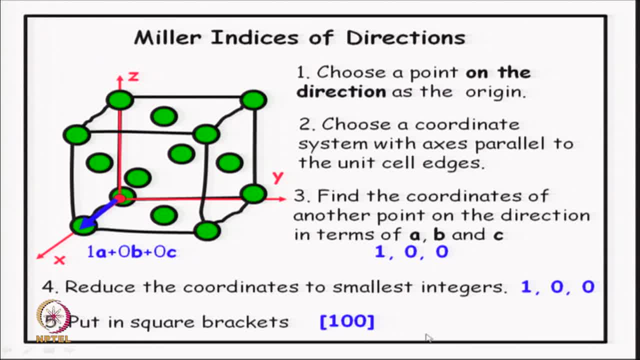 it with commas, but in the Miller indices I am not using any commas. So this is a useful convention. unless and until we have a 2 digit Miller indices for one of the component, if it is only 3 numbers, we write them without any commas, and it is. 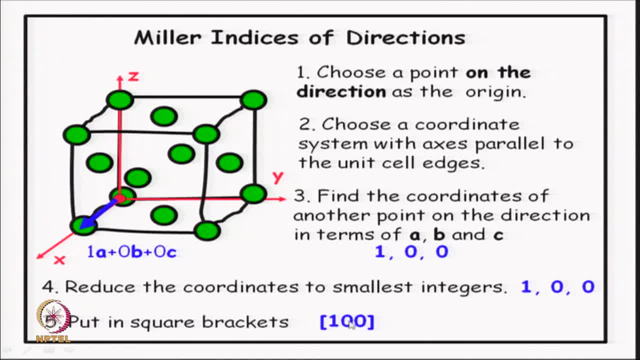 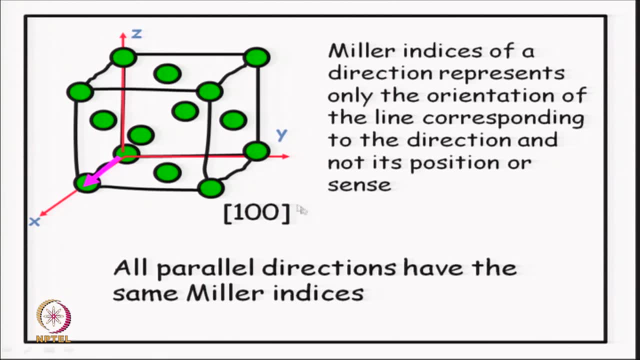 understood that the first number is with respect to the x axis, the second one with respect to the y and third one with respect to z. So let us look at some more examples now. before looking at those examples, one more point. So, Miller, indices of a direction represents only the orientation of the line, not its particular. 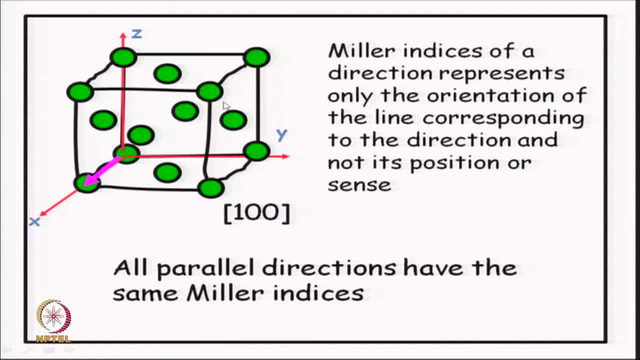 position in the space Or also its sense. so I already told that not only the positive x axis but the negative x axis will also be represented by 100 if we do not really want to distinguish positive and negative, that is to say if we are only interested in the line, not in the sense and 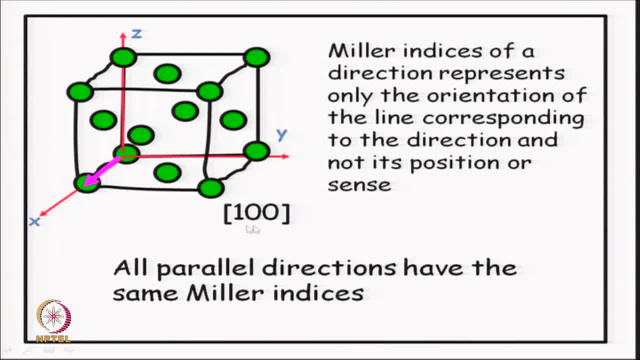 in Miller indices that is usually the case- then 100 represents the entire x axis. not only that, Because what we said about freedom of choosing the origin- if we had parallel lines somewhere here, then I can again choose my origin here and this will become my x axis. or I can choose. 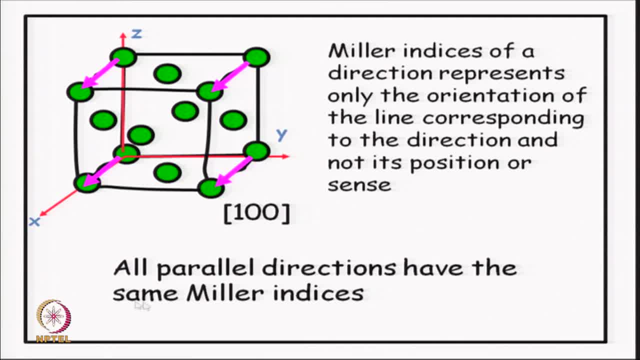 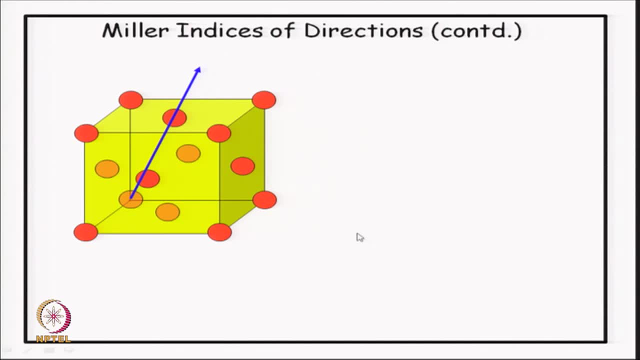 my origin there and this will become my x axis. So all parallel directions have the same Miller indices. let us now look at some more examples. So let us look at this point as my origin and axes along the unit cell edges. with respect, 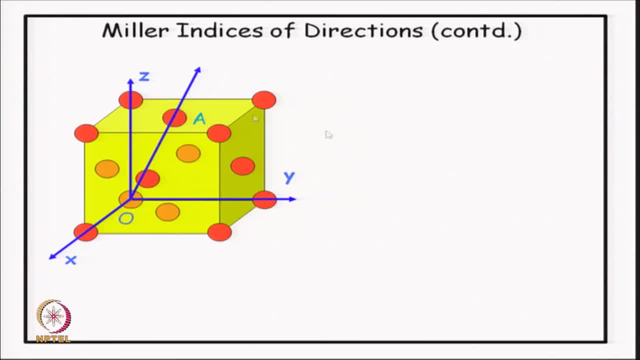 to this coordinate system. I now write the vector OA so you can see, to reach OA I have to go a by 2 steps along x, a by 2 steps along y and then c step along z. So OA, the vector OA, is half a plus half b and 1 times c. 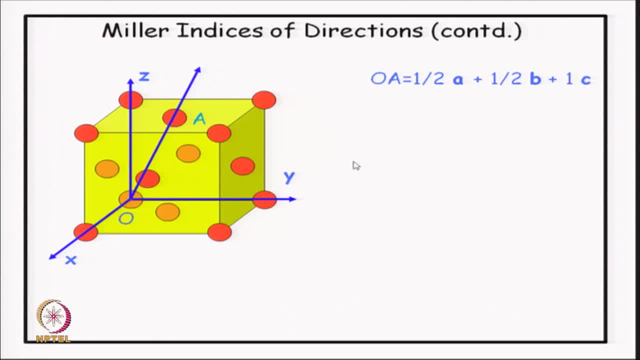 So the coordinates which we will use in the Miller indices in terms of a, b and c are half half and 1.. Now I will use the cancelling of fractions, step which we did not require in the previous one. In the case of 100, we did not require that. 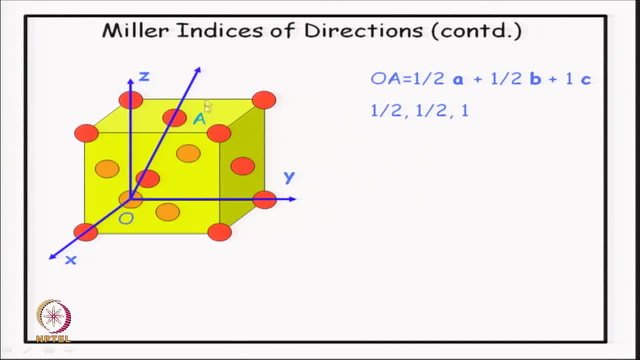 But now, in the case of half half 1, we will not call this direction half half 1, but we will simply multiply by 2 all these 3 numbers to get 1, 1, 2, and of course I put them in the square bracket which we have agreed upon to use as a convention for directions. 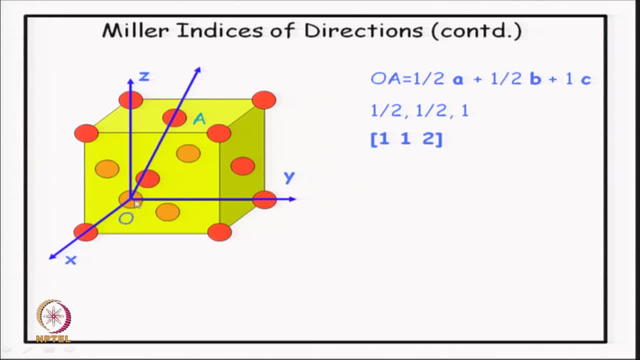 So the OA direction, not just the OA vector But the entire OA direction, Will be represented by this Miller indices 1, 1, 2.. One more example: let us look at this black direction. Now, of course I have to choose the origin on the black line, and that freedom is there. 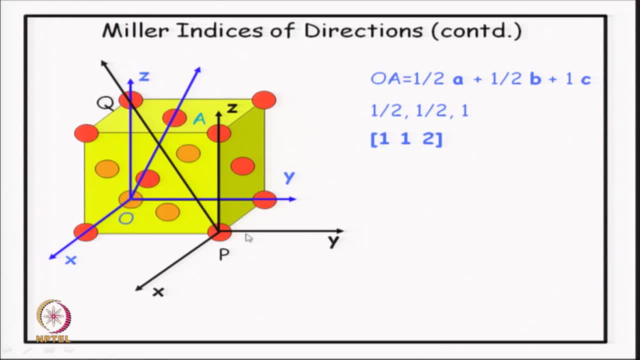 So I shift the origin to this point p on the black line. You can note that when I have shifted the origin I have kept the axes parallel, So we can see that. So we have the freedom to choose our origin anyway. 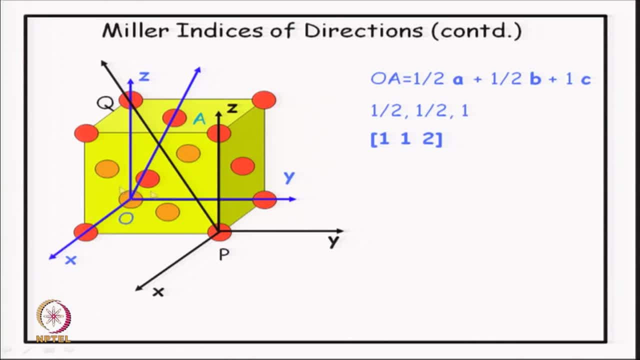 But in a given problem, once we have a specified the orientation of the axes, that orientation cannot change. So the xyz in the new, with the new origin, is exactly parallel to the xyz before. The black xyz is parallel to the blue xyz. So now let us try to index this direction along pq. 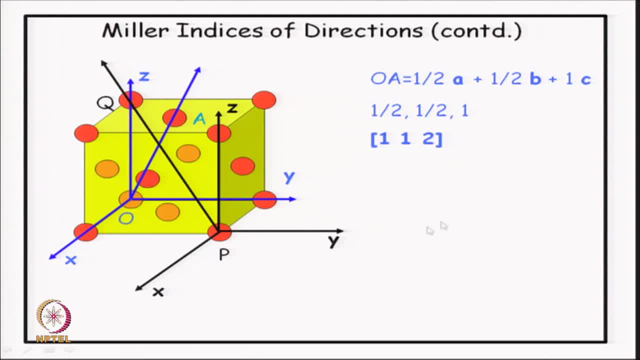 Which is one of the body diagonal. So if we want to look at this pq, So we will start with p and you can see that Now I have to take a minus 1 step along x, one step along y and one step along z to reach. 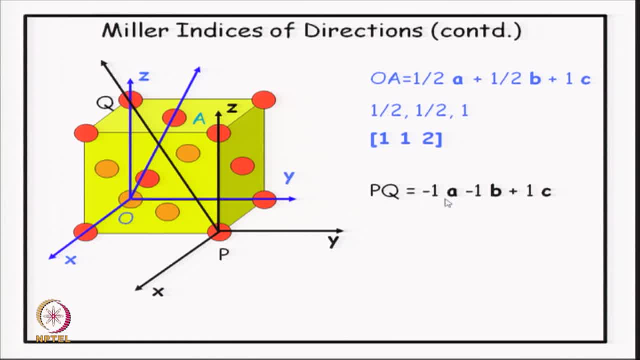 q. So the pq vector is minus 1 a, minus 1 b and 1 c. So the pq vector is also on pq. So now I have to find x, So I have to find. So the components are minus 1, minus 1, 1 in terms of a, b and c. 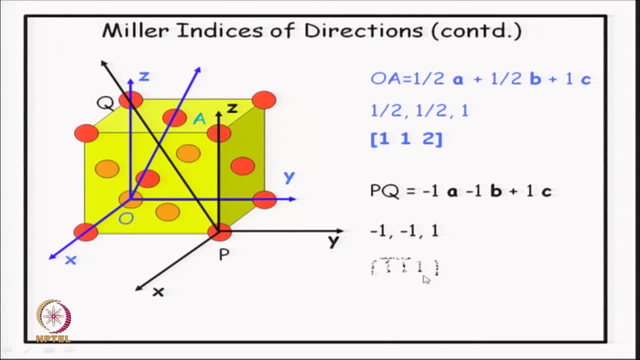 Now I write this in a square bracket with one additional convention: that the negatives are written as bars over the number instead of on the side, as in useful mathematics. in the Miller indexing notation a bar above the number represents negative quantity, So and it is read also as bar instead of minus 1.. 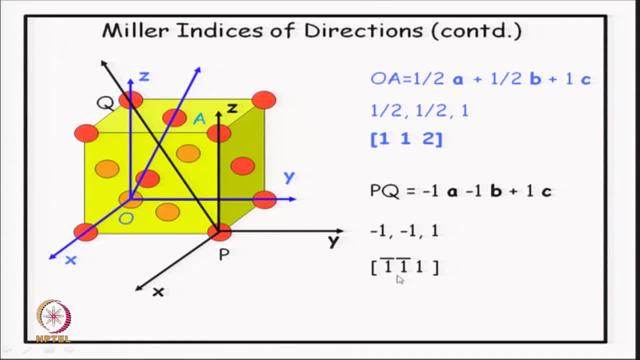 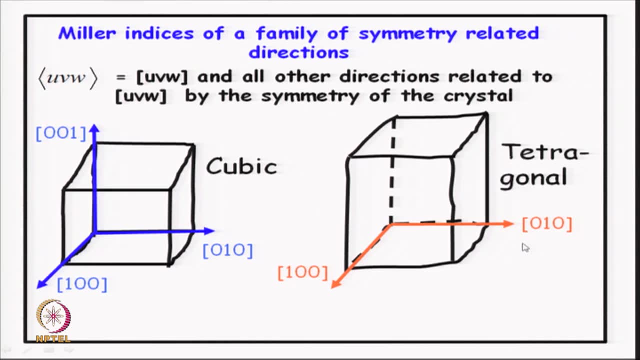 So we will call this direction PQ as bar 1, bar 1, 1.. Let us now take so the negative steps are shown as bar over the number. Let us now take So the negative steps are showed as bar over the number. 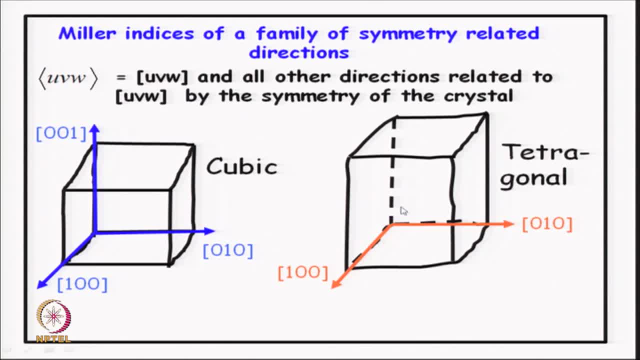 Let us now take. So the negative steps are shown as bar over the number. Let us now take. Now look at another convention which is used many times. we are not interested in just one direction, because we have talked about the symmetry in the crystal, and crystals can. 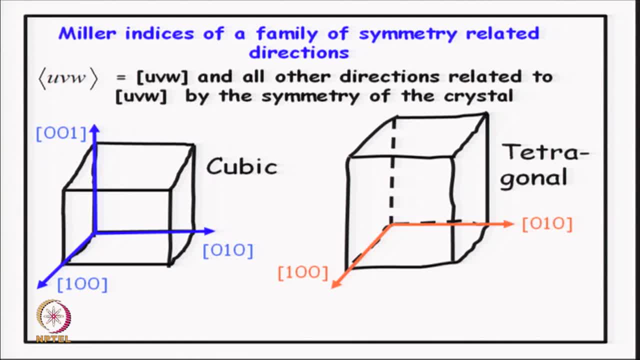 have symmetry, and symmetry relates many directions, So many directions become equivalent because of the existing symmetry of the crystal. So, for example, if you take a cubic crystal, so all the edges of the cube are equivalent by the cubic symmetry. So if we index the edge along x axis, it will be 100, if we index along the y axis, 010. and 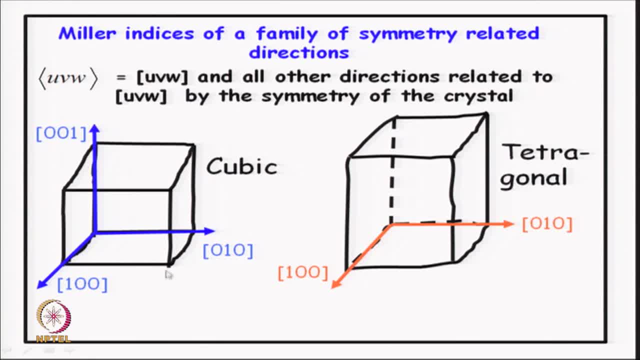 index along z axis 001.. But suppose I am not interested in the specific direction. I just want to talk about the cube edges, for all directions along the cube edge, which are equivalent by symmetry. Then there is a new notation That you can put the Miller index of any one of them in an angular bracket. 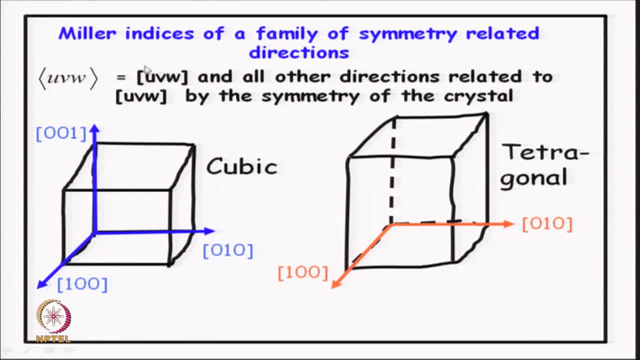 So an angular bracket, UVW means the specific direction UVW and all other direction related to UVW by the symmetry of the crystal. and it is important that when we are using this notation we have to know which crystal system we are talking about, because different crystals 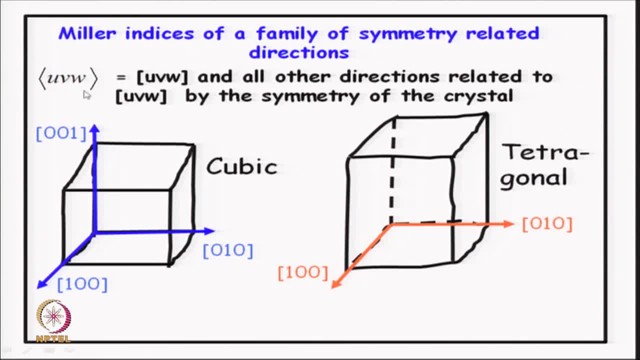 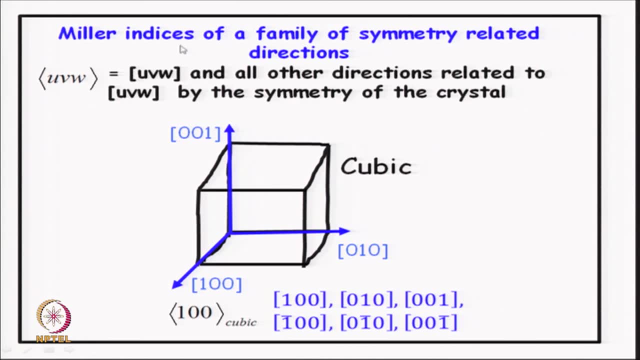 will have different directions, Different symmetry, and the symbol will mean different things. We will show you this with the help of cubic and tetragonal examples. So let us look at first the cubic. So in the Miller indices of cubic crystal, the 100 direction is equivalent to 010, 001. 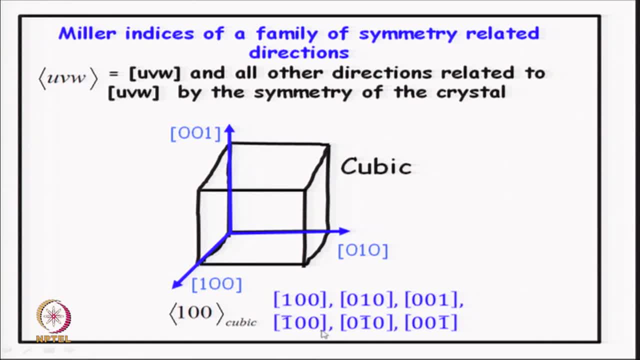 as well as if we take the negatives Minus bar 100, 0 bar 10 and 00 bar 1, so the all 6 directions are equivalent by the cubic symmetry. So if we simply write 100, if I pick any one of them, I have picked up 100, you could have. 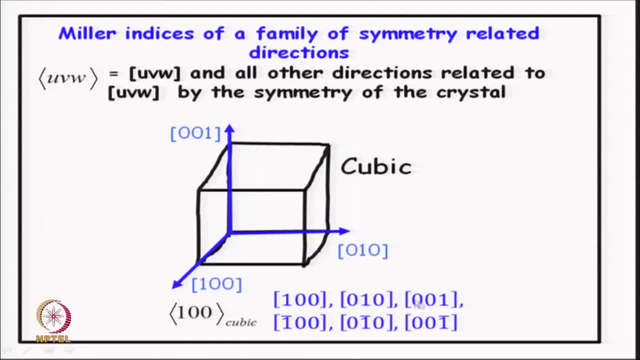 picked up 010 or 001, any of these, 6.. So any member of this direction. this is a family of 6 members. Okay, This is a family of symmetry related directions And I pick up any member of the family to represent the entire family.